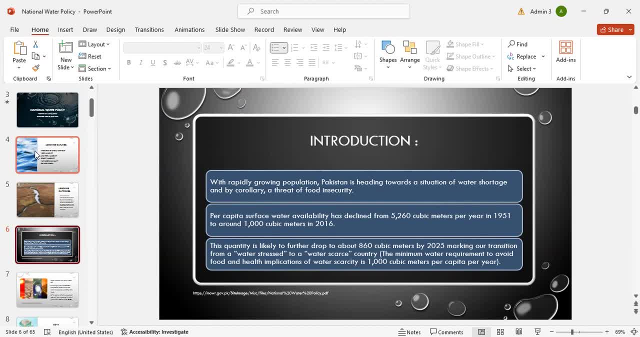 1,000 cubic meters in 2016.. This quantity is likely to further drop to about 860 cubic meters by 2025, marking our transition from a water stressed- as Pakistan is on 15 number on water stressed country to a water secrased country. The minimum water requirement to avoid food and other health implications is approximately 1,000 cubic meters per capita a year. We know that by the end of the year, the water level, the amount of water that can be utilized to reduce the fragrant and the amount of water that you can use to survive, will be very high. 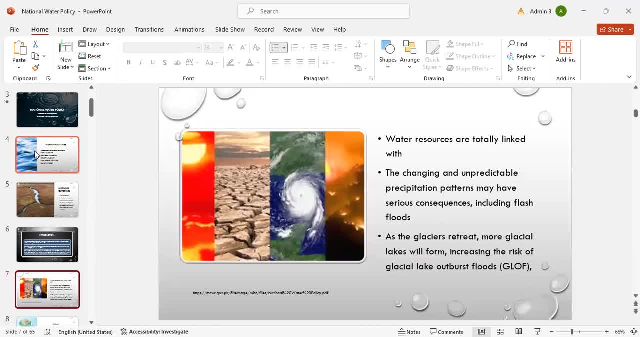 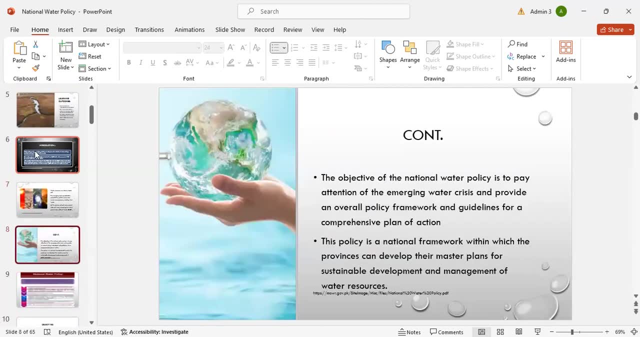 Water resources are also linked with the changing and unpredictable precipitation patterns. The changes in the water rate may have serious consequences, including flash floods, as more Glacial lags will form, increasing the risk for outbursts and landslides. The results of these studies are as follows. 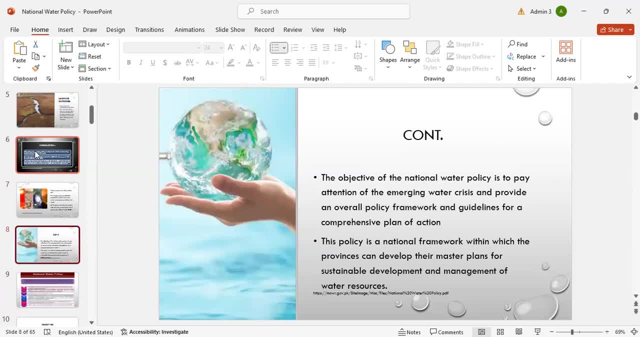 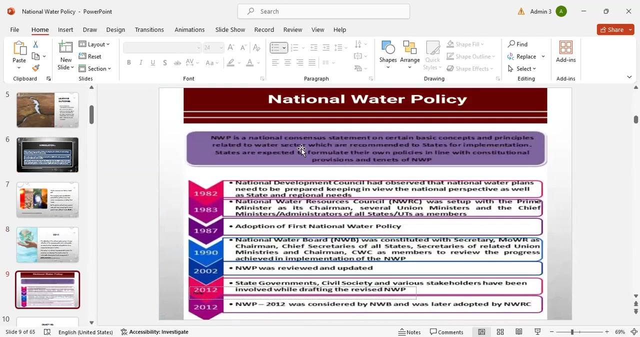 Slide 4.. the national water policy is to pay attention of emerging water crisis and provide an overall policy framework and guidelines for a comprehensive plan of action. This policy is national framework within which the provinces can develop their master plans for sustainable development and management of water resources. This picture showing the evolution in the national water: 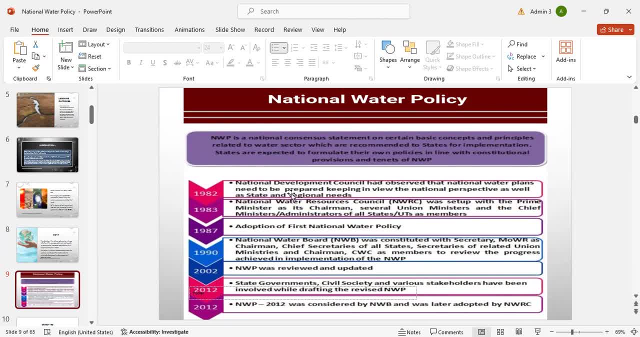 policy, as in 1982, National Development Council was developed, and then in 2002, national water policy was reviewed and updated, and then 2012, national water policies. 2012 was considered as a national water board and was later adopted by national water reserve national water reserve council, and then it is again reviewed in 2018.. 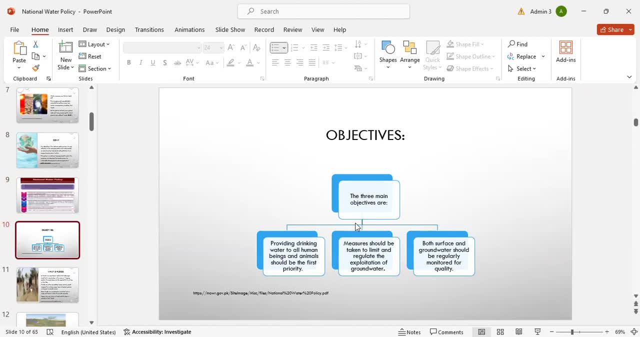 The objective of this policy. there are three main objectives. these are: providing drinking water to all human beings and animals should be the first priority. and second objective is major- should be taken to limit and regulate the exploitation of the ground water. The second objective is major, should be taken to limit and regulate the exploitation of the ground water. 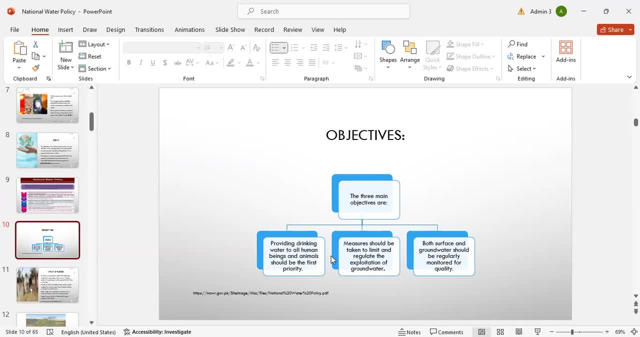 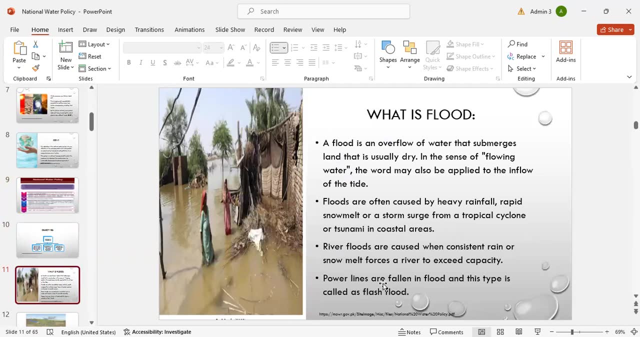 and third objective is: both surface and groundwater should be regularly monitored for quality. What is a flood? A flood is an overflow of water that submerges land that is usually dry. In the sense of flowing water, the word may also be applied to inflow of the tide. 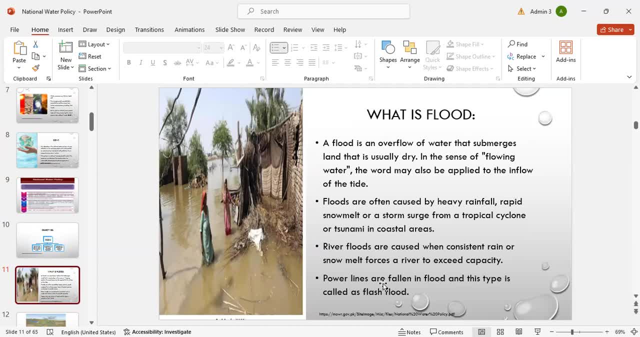 Floods are often caused by heavy rainfall, rapid snowmelt or a storm surge from a topical cycle, cyclones or tsunamis. in coastal areas, River floods are caused when consistent rain or snowmelt forces a river to exceed capacity. Power lines are fallen in floods and this 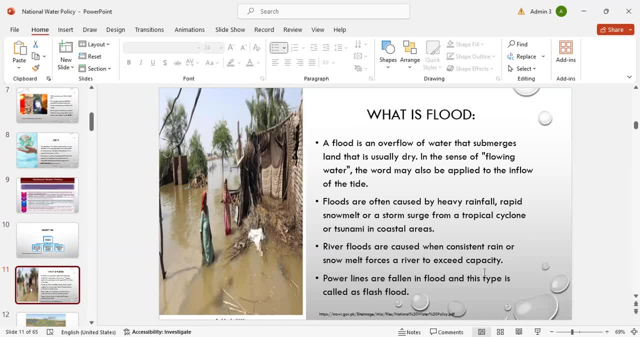 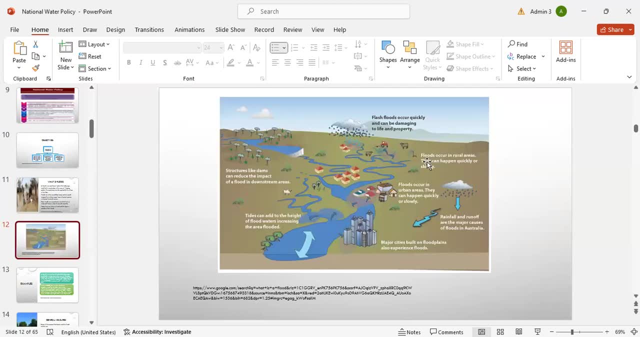 type is called a flash flood. This picture is showing that the development should be away from the flood areas- high risk areas. Then structures like dams can reduce the impact of the flood in the downstream areas and the tides can add to the height of the flood water. 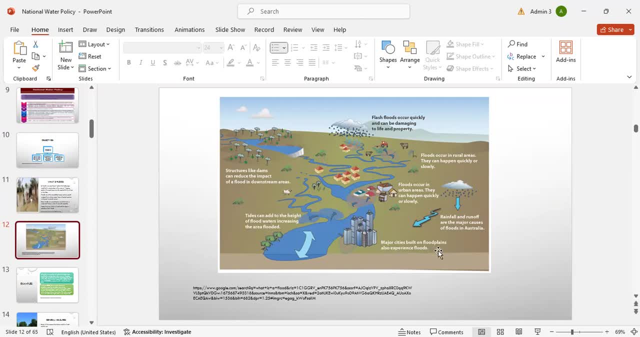 increasing the area flooded. Major cities built in the flood plains also experience floods, so these major cities should be away from high risk areas And floods occur in the urban areas. They can happen quickly or slowly. Rainfall and runoff are the major causes of the flood in Australia. 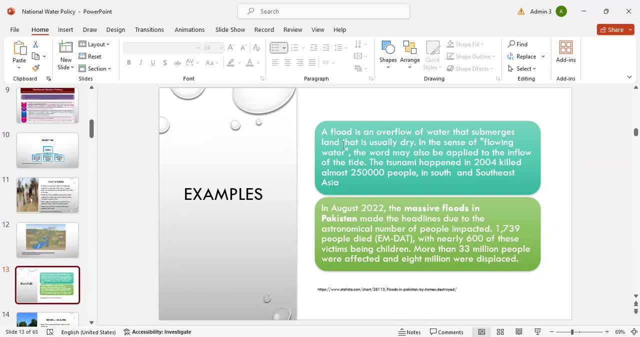 And the examples of the flood is an overflow of water that submerges land that is usually dry. in sense of flowing water, The word may also be applied to the inflow of tides. The tsunami happened in 2004, killed almost 2.5 lakh people in South and Southeast Asia In. 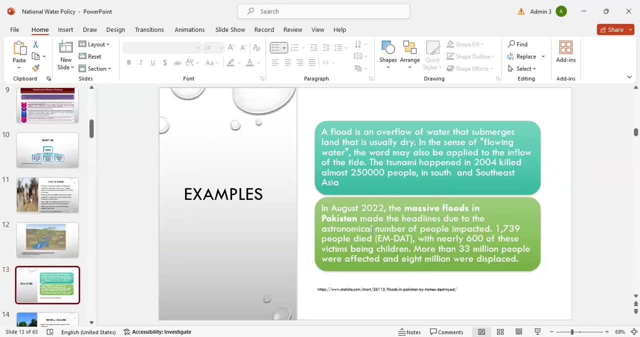 August 2022,. the massive flood in the Pakistan region caused a flood in the southern part of Pakistan made the headlines due to the astronomical number of the people impacted: 17, 1739 people died, with nearly 600 of these victims being children- More than 33 million. 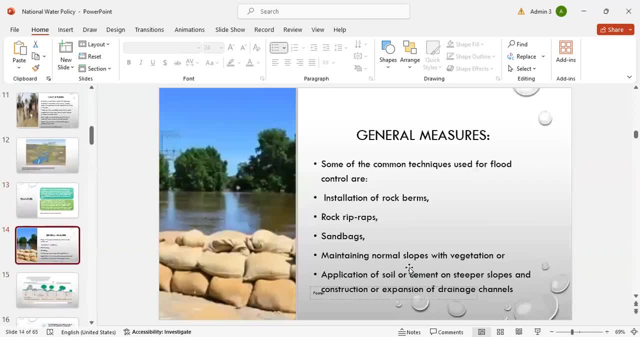 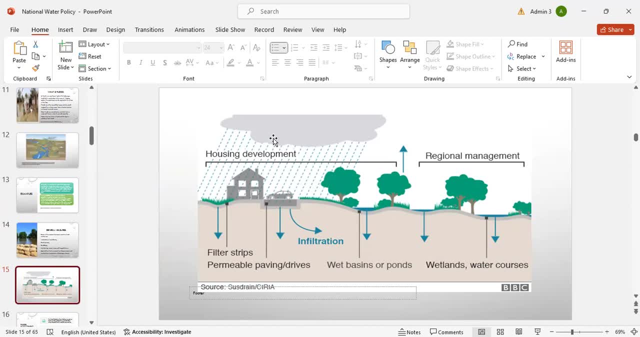 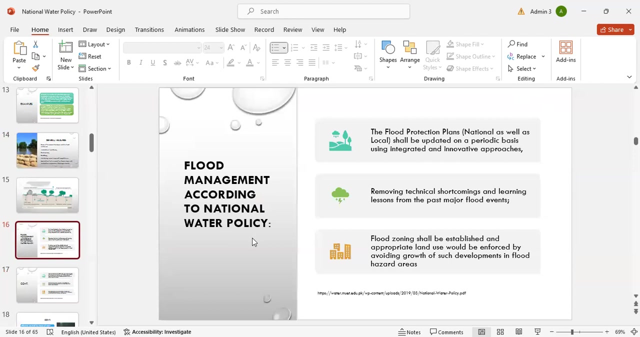 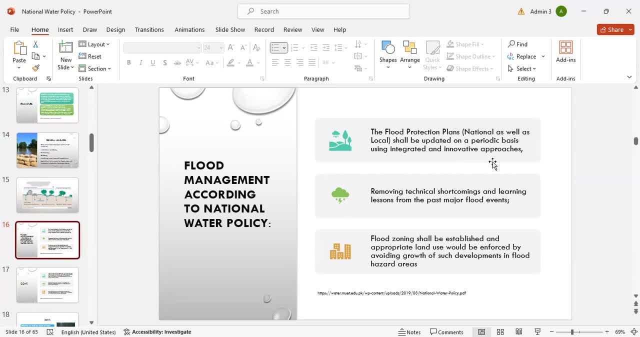 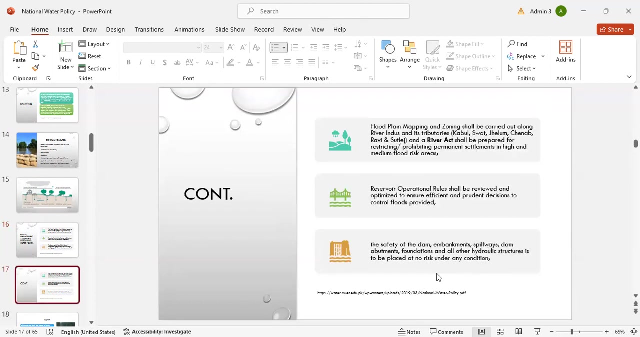 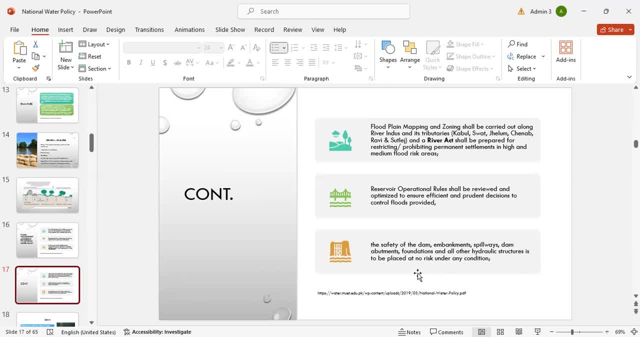 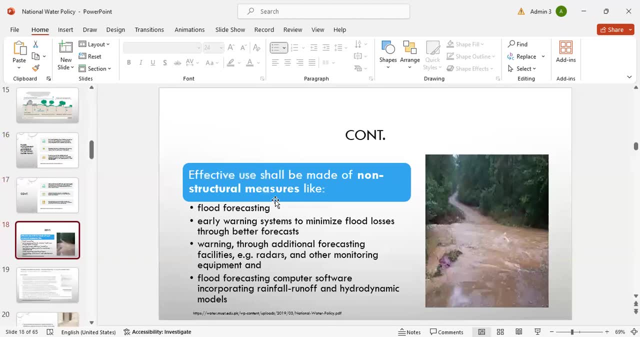 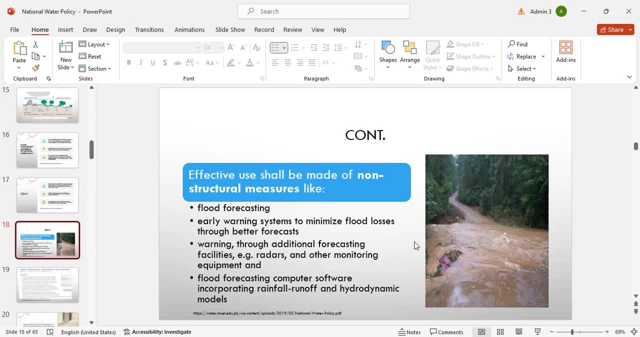 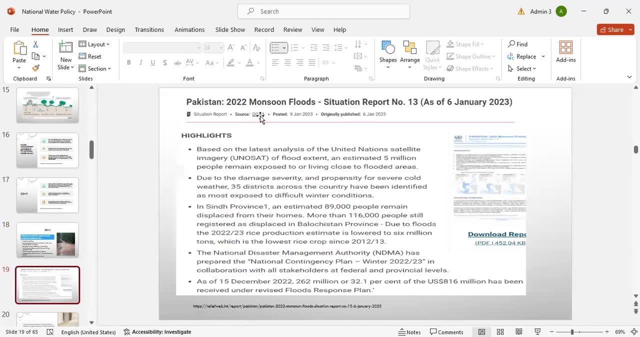 incorporating rainfall, runoff and hydrodynamic models. in pakistan, 2022 moonsault flood was the main highlight. this source is osha. based on the the latest analysis of united nations satellite imagery of the flood extent, an estimated 5 million people remain exposed to or living close to. 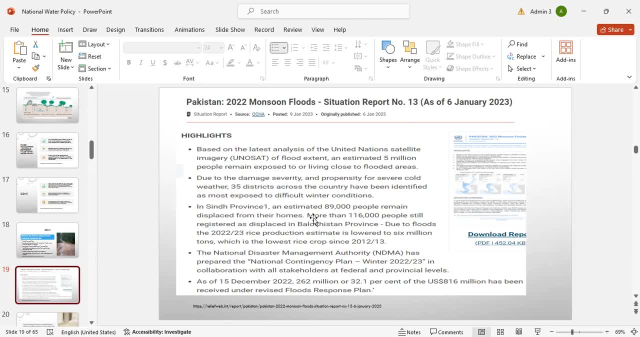 flooded areas, the sindh province and estimated 89 000 people remain displaced from their homes. more than 1 lakh and 16 000 people still register as a displaced in broochistan province. due to flood in 2022, 23 rice production estimate is lower to the 6 million tons, which is the lowest rice crop. 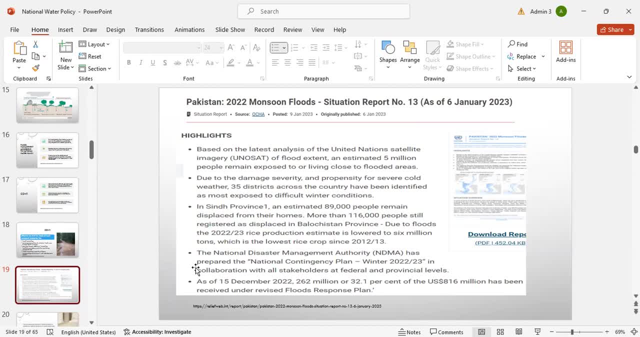 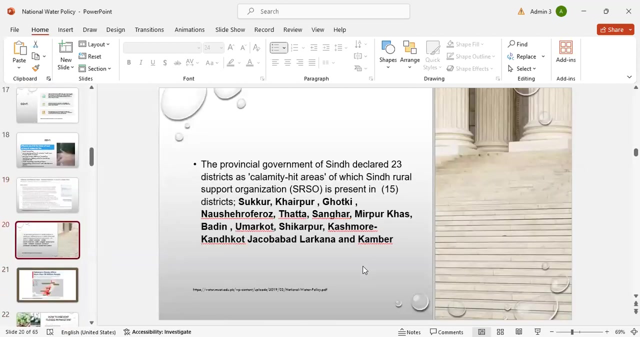 since 2012.. the as the 15th of december 2022, 262 million or 32.1 percent of the u uh us dollar 8 116 million has been received under the revised flood response plan. the provincial government of the cindy clear 23 district, as a climate heat areas, obviously in 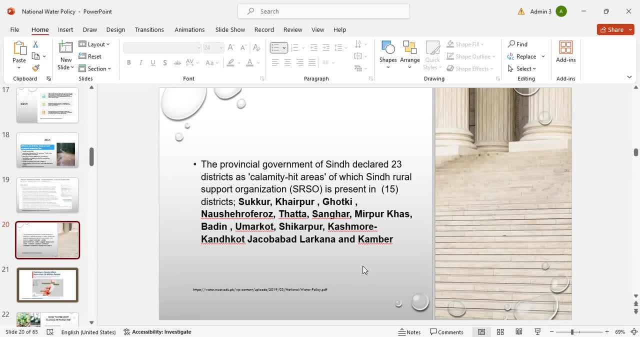 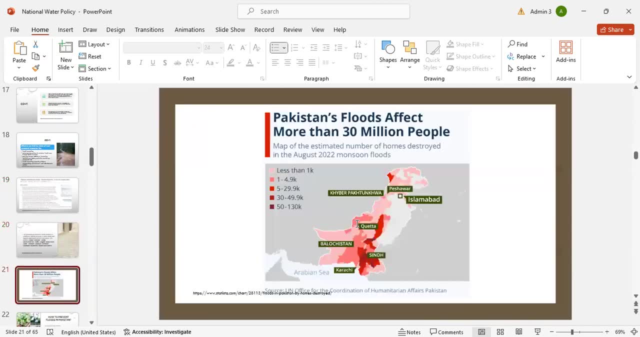 the rural sport organization is present in 15 districts. these include sakkar, harper and larkana, camber and others. pakistan's flood affected more than 30 million people. this picture showing that the areas where the heavy flood and mild flood affect the peoples where heavy flood occurs in the sindh, in the areas of especially the areas of sindh, and also in the. 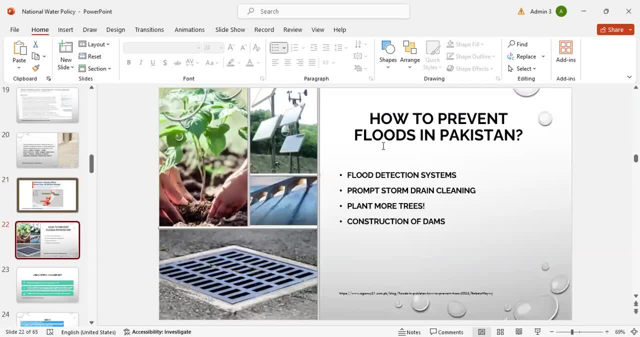 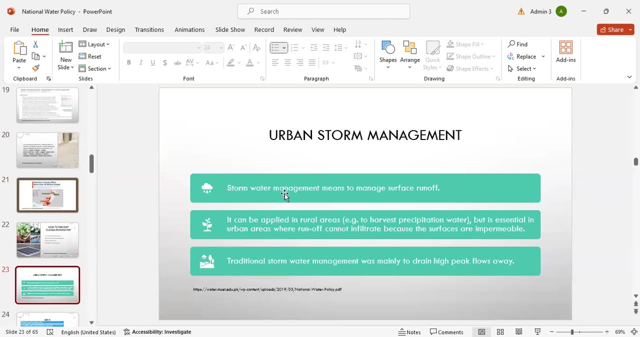 blochistan. how to prevent flood in india. how to prevent flood in india. how to prevent floods in the pakistan? flood detection: there should be flood detection systems. promote storm drain, cleaning, plant mode freeze and, by construction of dams, urban storm management. storm water management means to manage surface runoff. 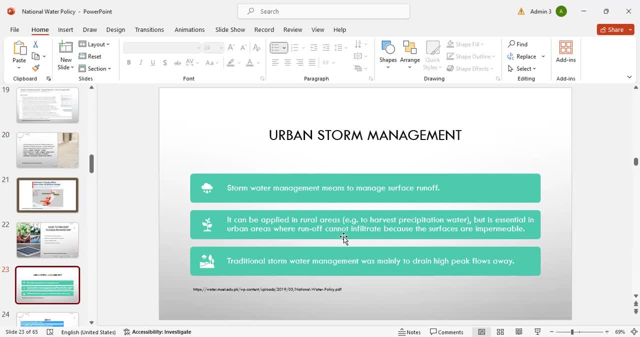 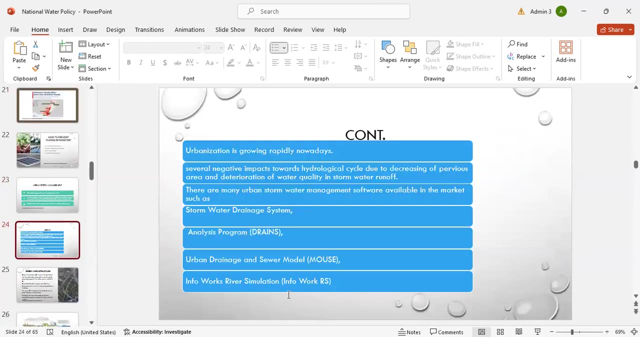 it can be applied in rural areas to harvest precipitation water but is essential in the urban areas where runoff cannot infiltrate because the surface are impermeable. predictor of the flood: impenable. traditional storm water management was mainly to drain high peak flow away. urbanization. as the urbanization is growing rapidly nowadays, several negative impact toward: 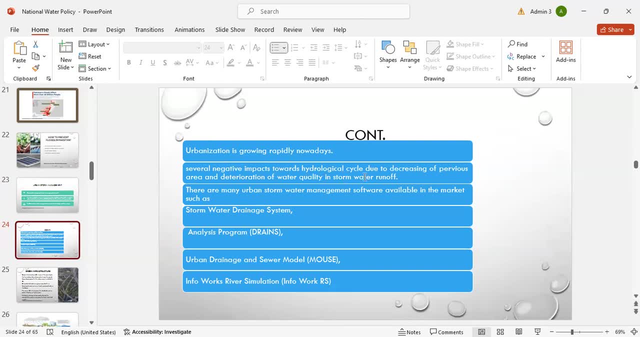 the hydrological cycle due to the decreasing of the previous areas, deterioration of the water quality in strong water runoff. there are many urban storm water management software available in the market, such as strong water draining system analysis program, urban drainage process drainage and saver model info work. river stimulation. 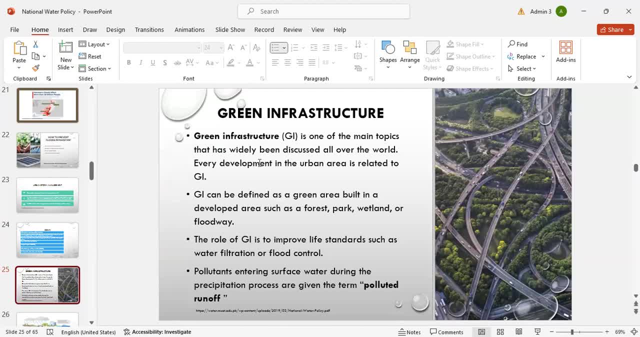 Green Infrastructure. Green infrastructure is one of the main topics that are widely discussed all over the world. Every development in the urban areas is related to green infrastructure. Green infrastructure can be defined as a green area built in and developed areas such as forests, parks or flood bays. 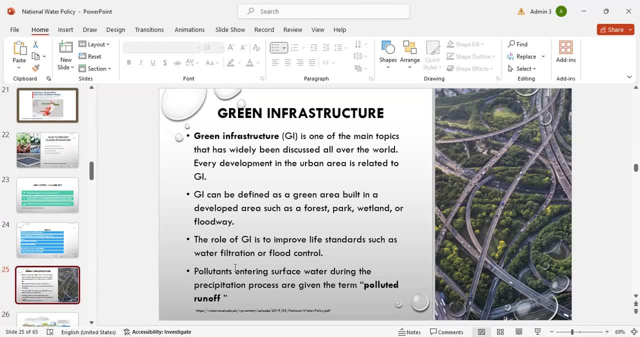 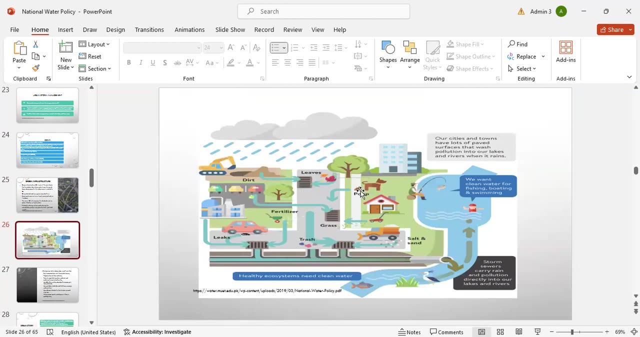 The role of the green infrastructure is to improve life standards, such as water filtration or flood control. pollutants entering in the surface water during the precipitation process are given the term polluted runoff. This picture system is showing that the ecosystem that need a fresh water, that water should. 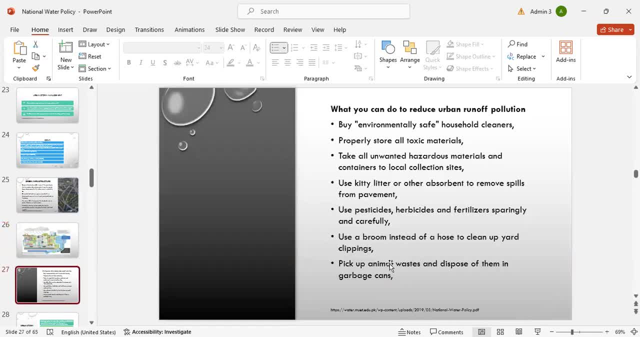 be prevented from the pollution. What we can do to reduce the urban runoff pollution By environmentally safe household cleaners, by properly storage all toxic material. take all the unwanted hazardous materials and containers to local collection sites. use kit liters or other absorbent to remove spills. 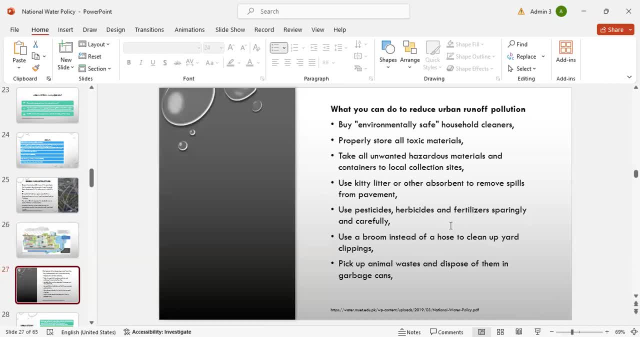 from the pavement. use pesticides, herbicides and fertilizers sparingly and carefully. use a broom instead of a hose to clean up yard clippings. pick up animal waste and dispose them in the garbage canes. Urban Storm Management Inventory. 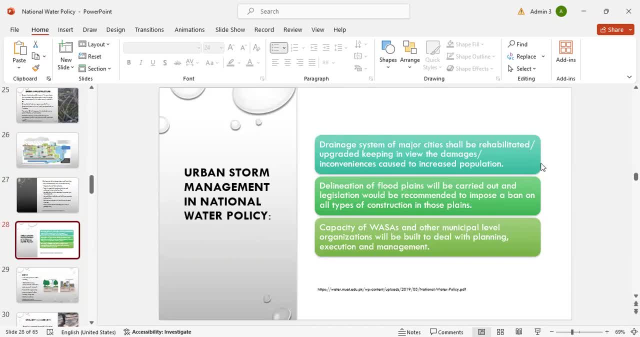 Drainage system of the major cities shall be rehabilitated, upgraded, keeping in view of the damages, inconveniences caused to increase population, delineation of the floodplains will be carried out and the legislation would be recommended to impose a ban on all types. 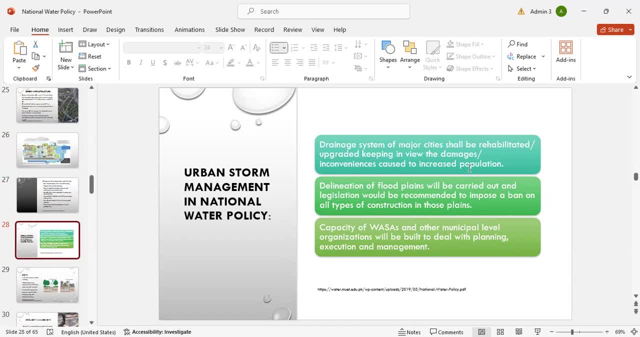 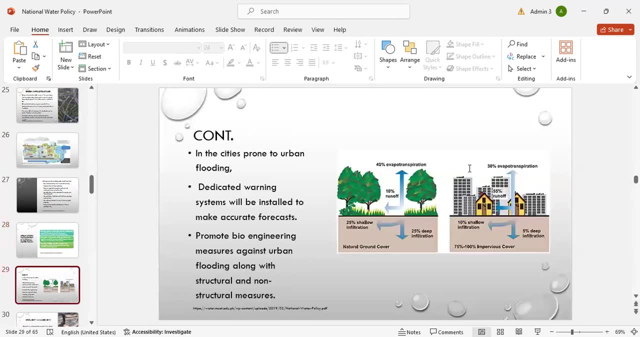 of construction in these plains. Capacity of VASAs and other municipal level organizations will be built to deal with planning execution and management. In the cities prone to urban flooding, dedicated warning systems will be installed to make accurate forecasts, promote bioengineering measures against urban flooding, along with 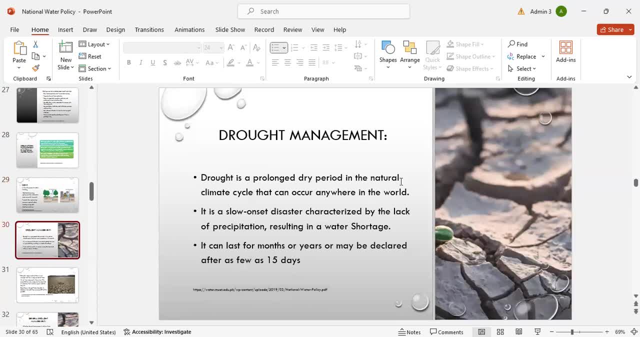 structural and non-structural measures. Draft Management Draft is a prolonged dry period in the natural climate cycle that occurs anywhere in the world. It is slowly onset A disaster characterized by the lack of precipitation, resulting in a water shortage. It can last for months or years, or may be declared after as few as 15 days. 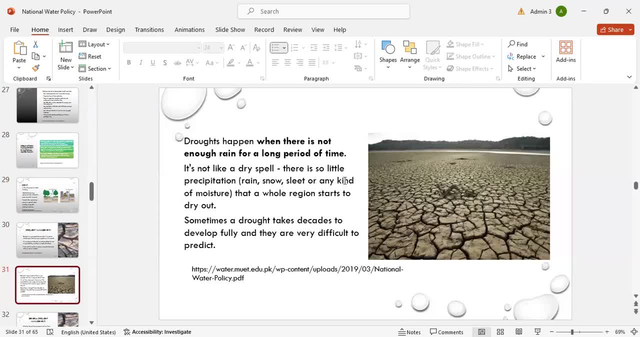 Drought happens when there is not enough rain for a long period of time. It is not likely a dry spell. There is so little precipitation- rain, snow, sleet or any kind of moisture- that a whole region starts to dry out. 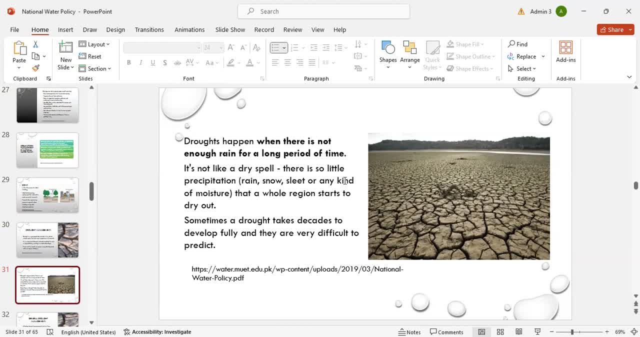 Sometimes a drought takes decades to develop fully or they are difficult to manage. It is not likely a dry spell. There is so little precipitation- rain, snow, sleet or any kind of moisture- that a whole region starts to dry out. 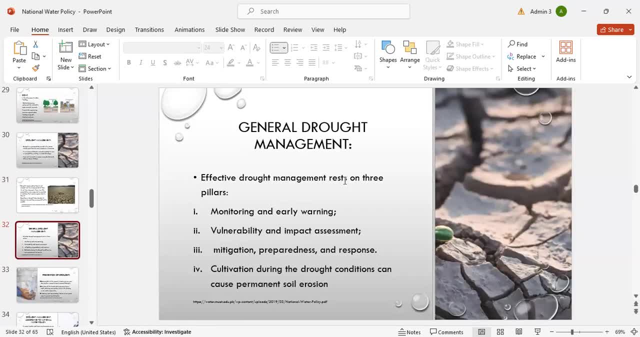 It is difficult to control by any means Draft Management. Effective draught management rests on three kinds of pillars: Monitor, early warning, vulnerability and impact assessment, Mitigation, preparedness, response and cultivation during the drought condition can cause permanent soil erosion. 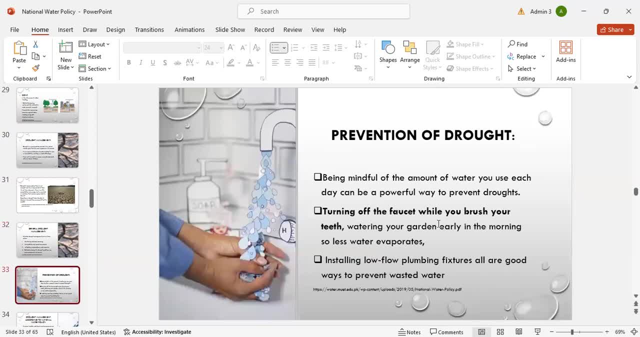 Prevention of Drought: Being mindful of the amount of water in your pipes: every day can be a powerful discussion on increasing soil concentration. Prevention of Drought: Be careful with water remaining on the accur. deeply Turn off the taps when you brush your teeth. watering your garden early in the morning so less water evaporates. installing low-flow plumbing fixtures: all are good ways to prevent wastage of water. 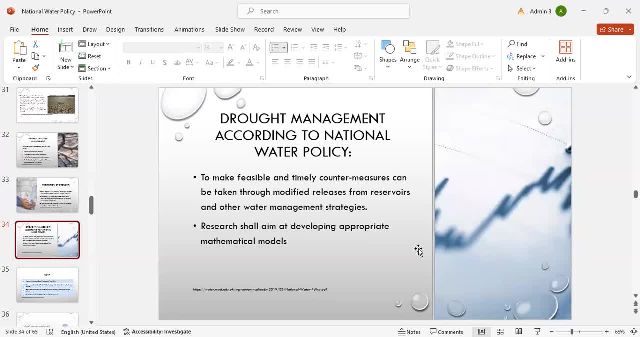 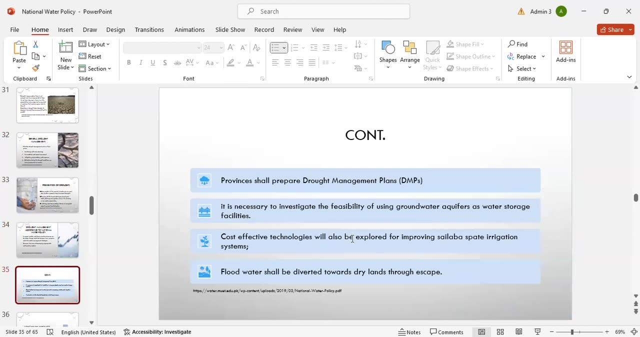 Road management according to national water policy. To make feasible and timely countermeasures can be taken through the modified releases from the reservoirs and other water management strategies. Research shall aim at developing appropriate mathematical models. Provinces shall prepare drought management plans. It is necessary to investigate the feasibility of using groundwater equal fire as a water shortage. 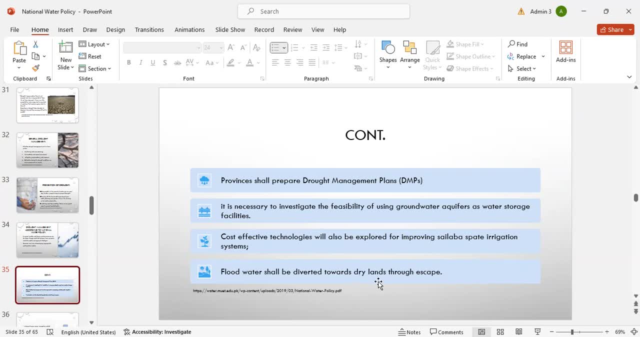 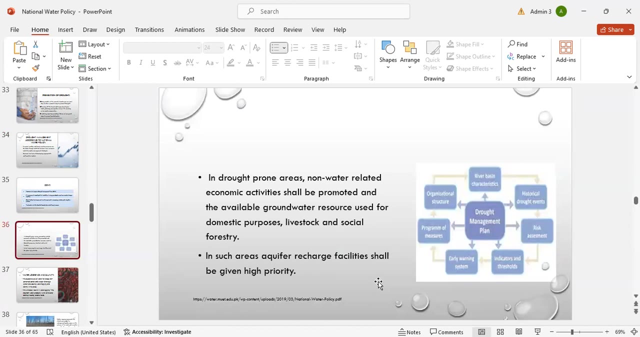 Facilities. cost-effective technologies will also be explored for improving Salaba spread irrigation system. A flood water shall be diverted toward dry land through escape. In drought-worn areas, non-water-related economic activities shall be promoted and the available groundwater resources should for domestic purpose, livestock and social forestry. 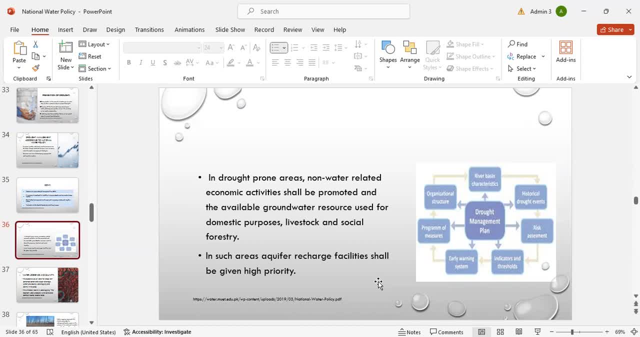 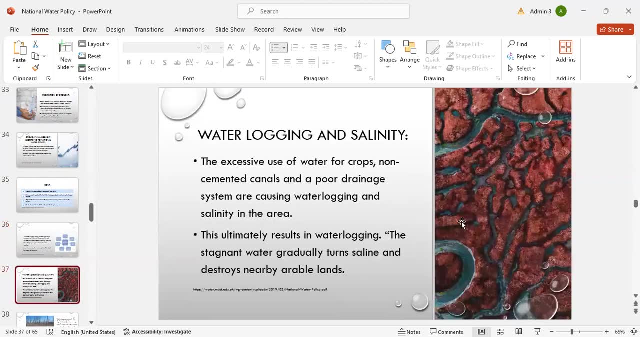 In such areas, equal fire recharge facilities shall be given at high priority. These are points for the management of the drought plan. Drought management plan. Water logging and salinity. The excessive use of water. The excessive use of water, The excessive use of water for crops, non-cemented canals and poor drainage systems are causing water logging and salinity in the areas. 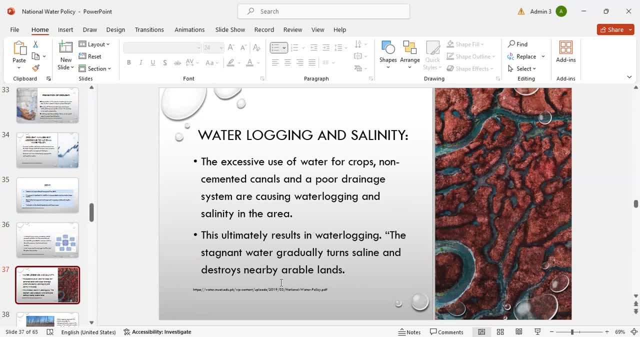 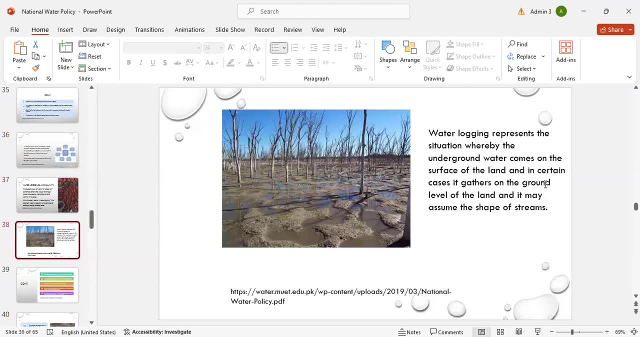 The ultimate result in water logging. Thus stagnant water gradually turns saline and destroys nearby arable lands. Water logging represents the situation whereby underground water comes on the surface of the land and in certain cases it gathers on the ground level by the land and it may assume the shape of the streams. 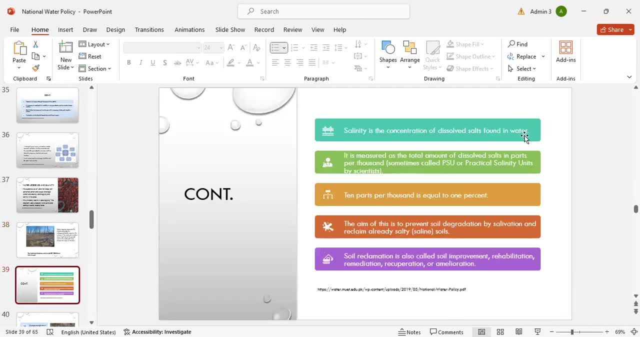 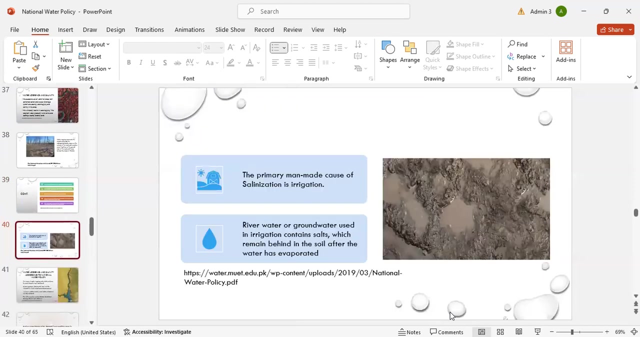 A condition that 회v coupled withடhe Salinity. Salinity is the concentration of dissolved salt found in the water. It is measured as the total amount of dissolved salt in the world. Ô Ô Apa ów Au υ called the soil. improvement, rehabilitation, remediation and amelioration. 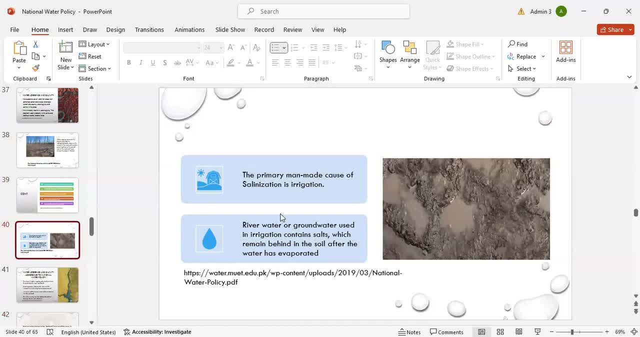 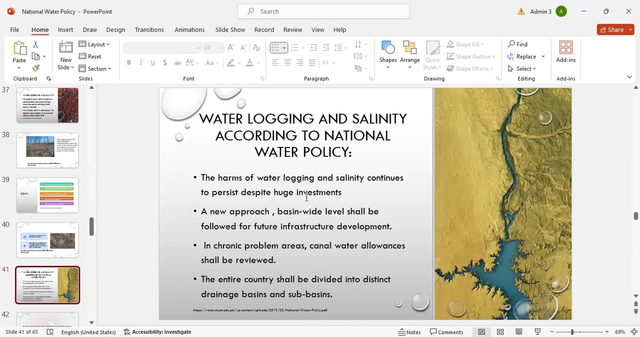 The primary man-made cause of the salinization is irrigation. River water or groundwater used in irrigation contains salts which remain behind the soil after the water has evaporated, Water Longing and Salinity. According to National Water Policy, the harm of water longing and 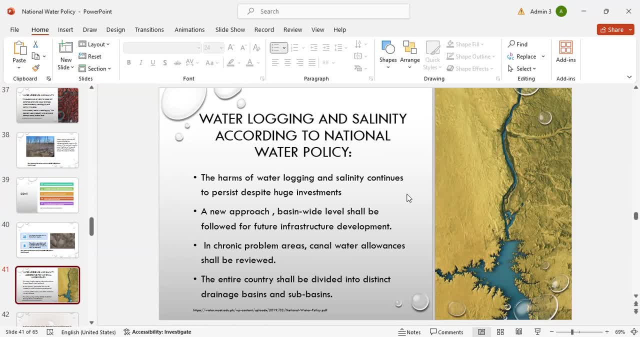 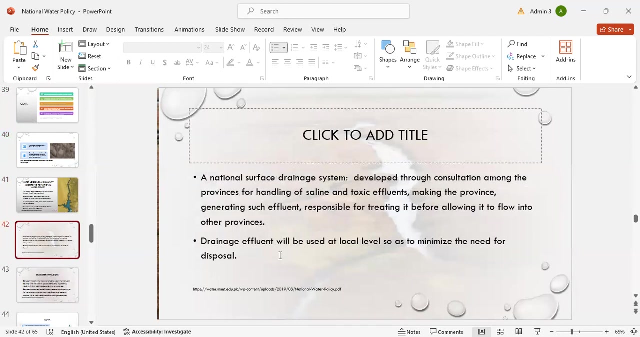 salinity continues to persist despite huge investment. A new approach, basin-wide level, should be followed for the future infrastructure development In chronic problem areas. canal water allowance shall be reviewed. The entire country shall be divided into distinct drainage basins and sub-basins. The National Surface Drainage System developed. 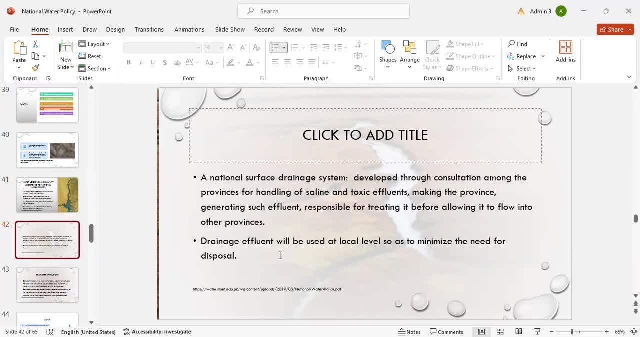 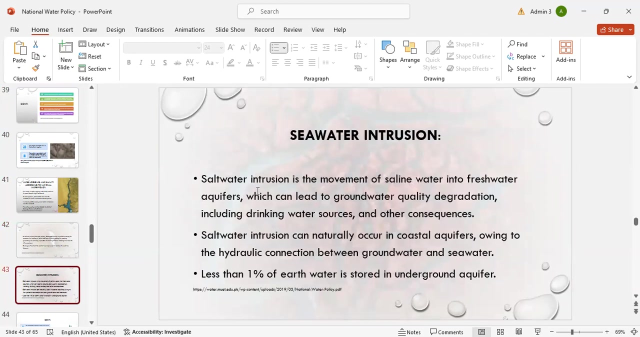 through the consultation among the provinces, for handling for sludge and toxins. The National Surface Drainage System, developed through the consultation among the provinces, for handling for sludge and toxins. The National Surface Drainage System, developed through the collaboration among the provinces, for handling for sludge. 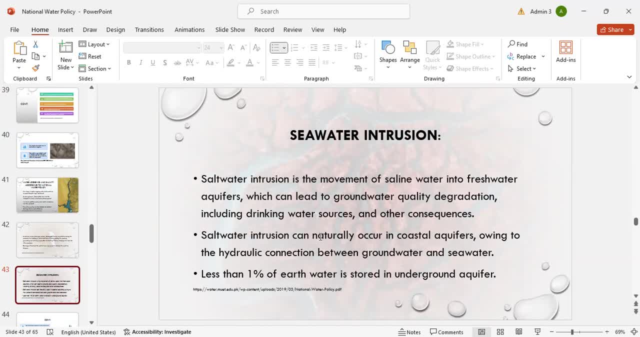 and toxins, A second road systemнаvel infrastructure and water resources, and other consequences. Saltwater intrusions can naturally occur in the coastal equivifiers owing to the hydraulic connection between the groundwater and sea water. Less than 1% of the earth water is. 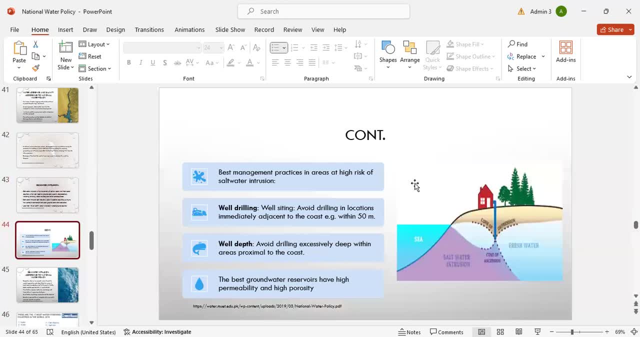 stored in underground equivifier. The best management practice in the areas at the high risk of saltwater intrusion are: well drilling, well sitting. avoiding drilling in the location immediately adjacent to the coast, for example, within 50 meters well depth. Avoid drilling excessively deep within the areas. 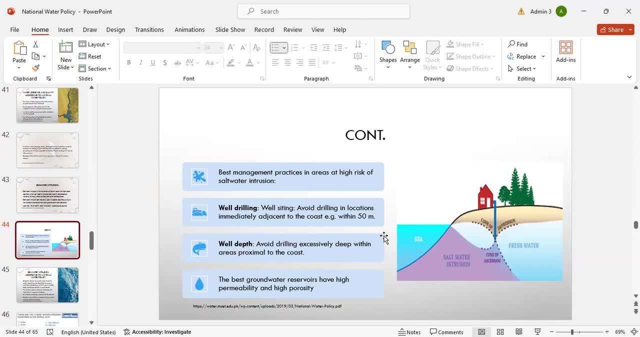 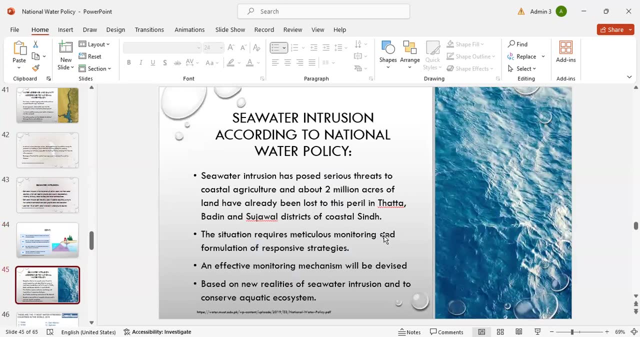 proximal to the coast And the best groundwater reservoirs have high permeability and high porosity. Seawater intrusion. according to national water policy, Seawater intrusion has posed serious threats to the coastal agriculture and about 2 million acres of the land have already been lost in this peril in Thatta. 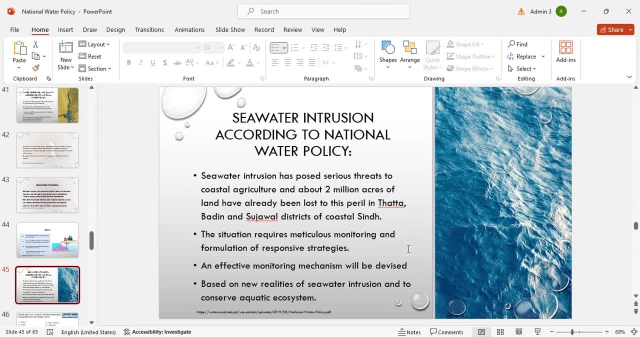 Badin Sajawal district of the coastal. The situation requires meticulous monitoring and formulation of the response strategies, and effective monitoring mechanism will be devised based on new realities of the seawater intrusion and to conserve equative ecosystem. These are the 17 most important factors. 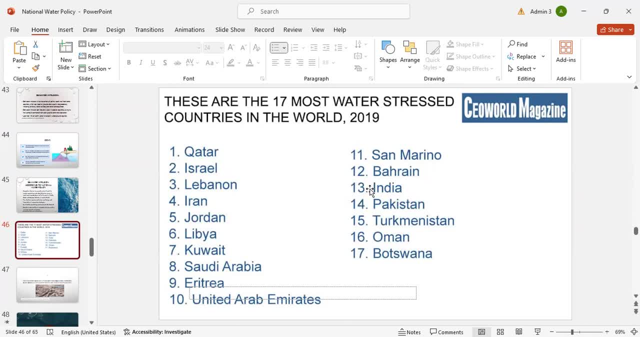 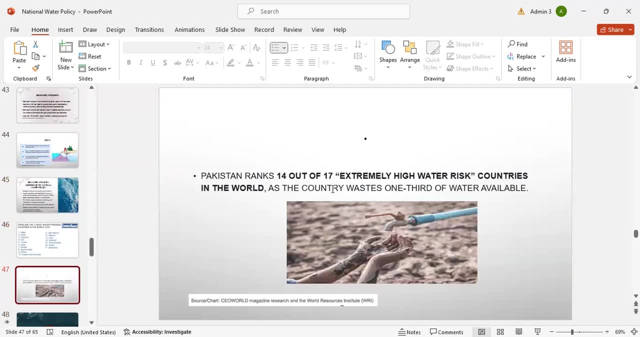 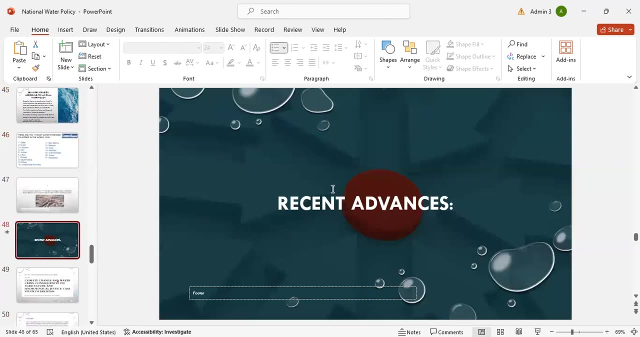 in the most water-stressed countries, where Pakistan is on 14th number. Pakistan ranks 14 of the 17 extremely high water risk countries in the world, as the country weighs one third of the water that is available. Now, coming to the recent advances, 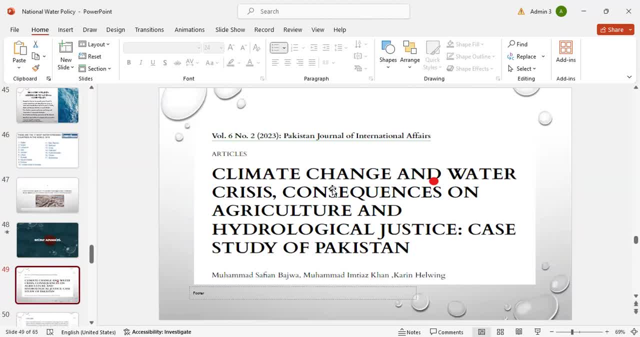 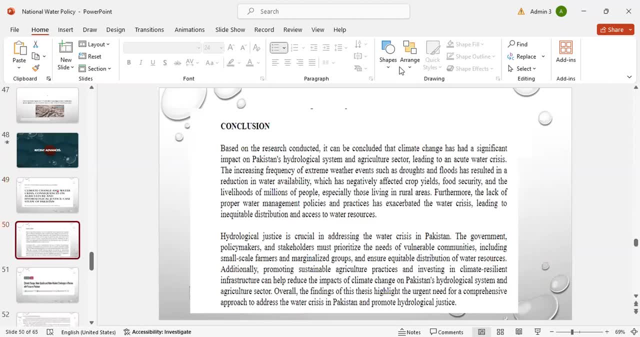 Our first article is Climate Change and Water Crisis: Consequences on the Agriculture and Hydrological Justice Case Study of Pakistan. Now the conclusion of this study is. based on the research conducted, it may be concluded that climate change has had a significant impact on Pakistan's hydrological system. 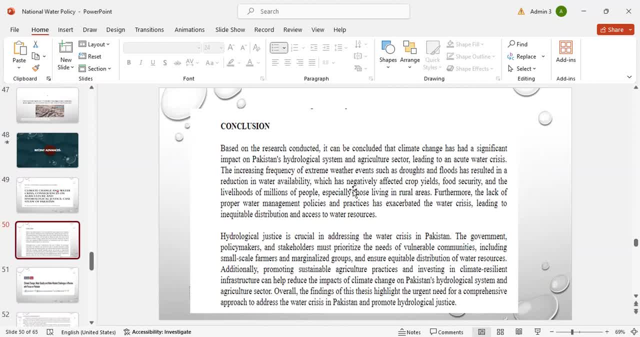 and agriculture sector, leading to acute water crisis. The increasing frequency of extreme weather events, such as drought and flood, had resulted in reduction in water availability, which has negatively affected crop yield, food security and livelihood for the millions of the people, especially those living. 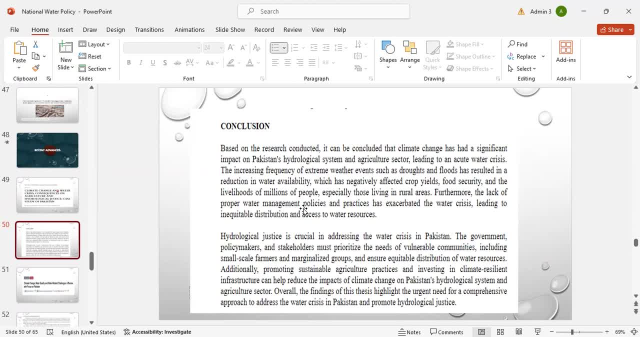 in the rural areas. Furthermore, the lack of the proper water management policies and practice has accelerated the water crisis, leading to inequitable distribution and access to the water resources. Hydrological justice is crucial in addressing the water crisis in Pakistan: The government, policymakers and stakeholders. 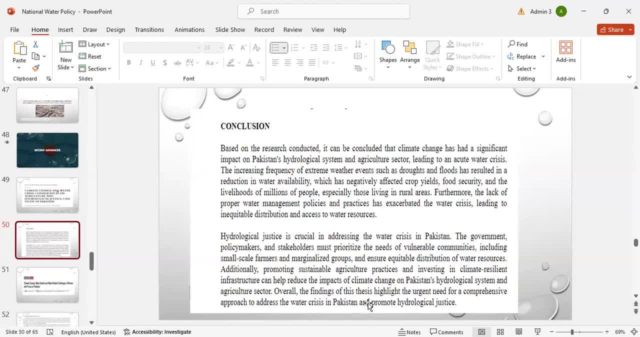 must prioritize the need of the vulnerable communities, including small-scale farmers and marginalized groups, and ensure equitable distribution of the water resources. Additionally, promoting sustainable agriculture practices and investing in climate resilient infrastructure can help reduce the impact of the climate change. in Pakistan, hydrological system and agriculture structure. 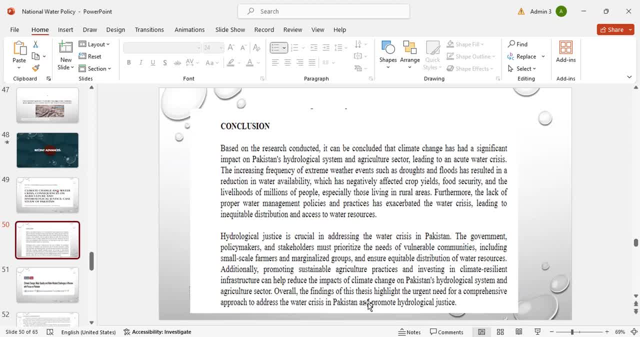 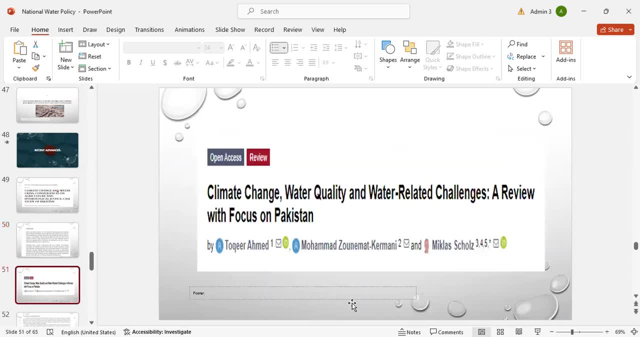 Overall, the finding of this thesis highlights the urgent need for a comprehensive approach to address the water crisis in Pakistan and promote hydrological justice. The second article is Climate Change, Water Quality and Water-Related Challenges: a Review with Focus on Pakistan. 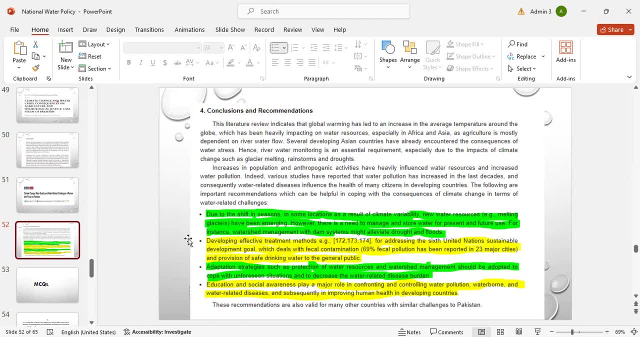 These are the main points of this literature review. Due to the shift in the seasons in some locations as a result of the climate variability, new water resources- melting glaciers- have been emerging. However, there is a need to manage and store water for present and future use. 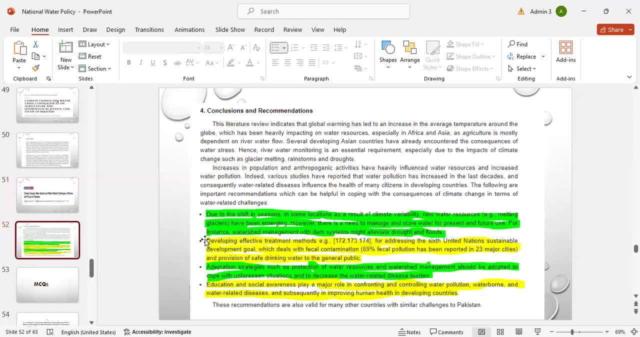 For instance, watershed management with dam system might alleviate drought and floods. Developing effective treatment methods, for example 172, 173, 174, for addressing the United Nations Sustainable Developing Goals, which deals with the fecal contamination: 69% fecal pollution has been reported in 23 major cities. 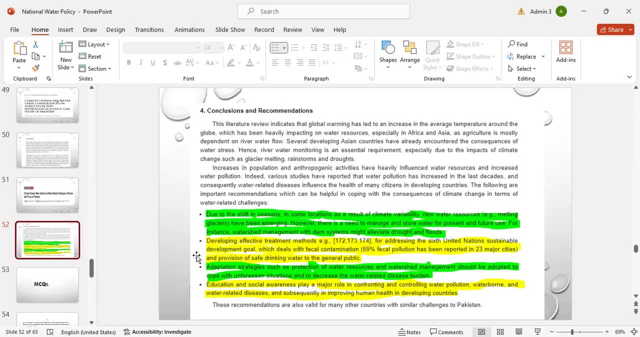 and provision of safe drinking water to the general public. Adaptation strategies such as protection of water resources and watershed management should be adopted to cope with the unforeseen situation, to decrease the water-related disease burden. Education and social awareness play a major role in confronting and controlling water pollution. 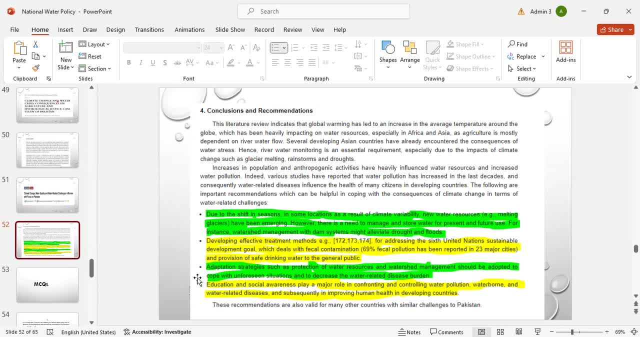 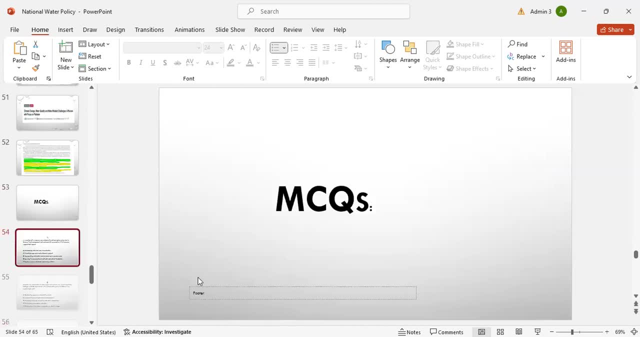 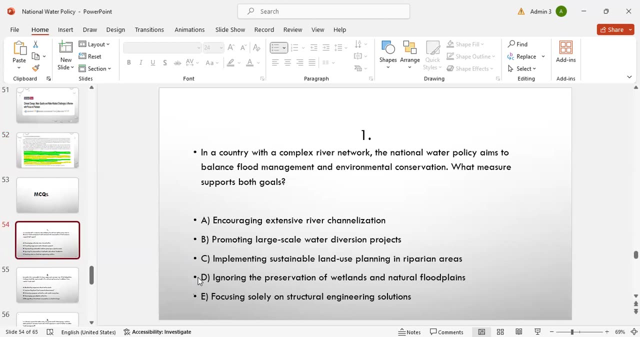 waterborne and water-related diseases and subsequently in improving human health in developing countries like Pakistan. So let's move on to our MCQ session First. MCQ is in a country with a complex river network, a national water policy aimed to balance flood management. 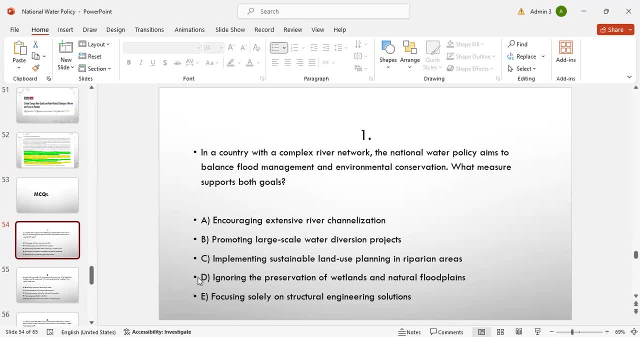 and environmental conservation. What will support the both goals? Option A- encouraging extensive river channelization. Option B- promoting large-scale water diversion projects. Option C- implementing sustainable land use planning in riparian areas. And option D- ignoring the preservation of the wetlands. 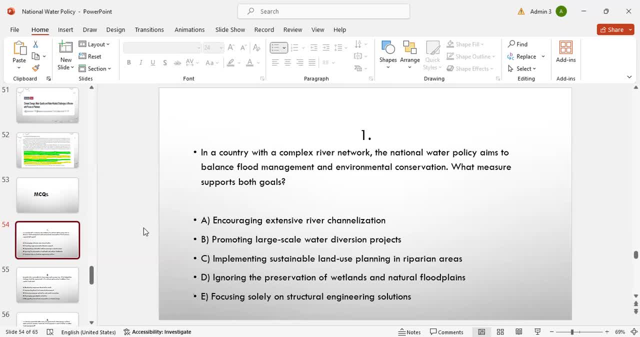 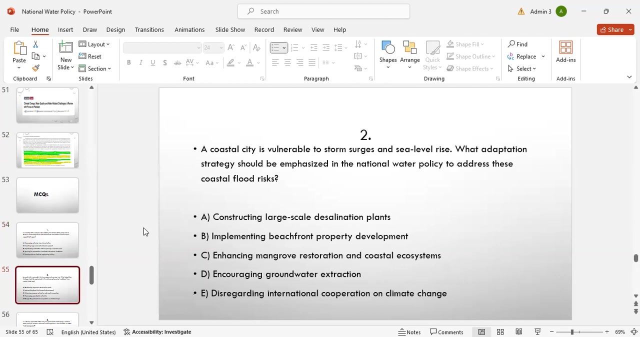 and natural floodplains. E is focusing solely on structural engineering solutions. B answer is option C: implementing sustainable land use planning in riparian areas. MCQ number two is: a coastal city is vulnerable to storm surges and sea level rise. 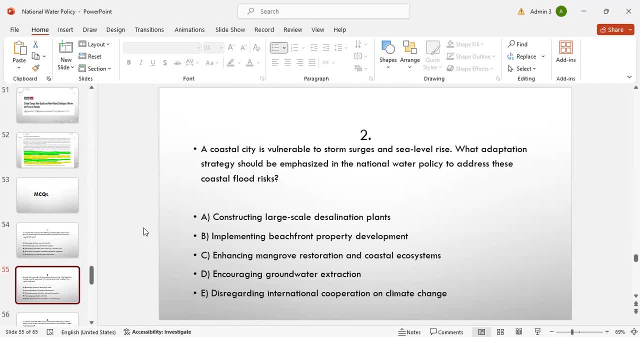 What adaptation strategy should be emphasized in the national water policy to address these coastal flood risks? Option A: constructing large-scale desalination plants. Option B is implementing beachfront property development. Option C is enhancing mangrove restoration and coastal ecosystem. 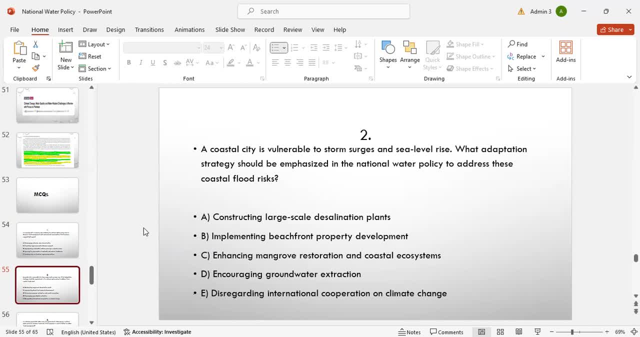 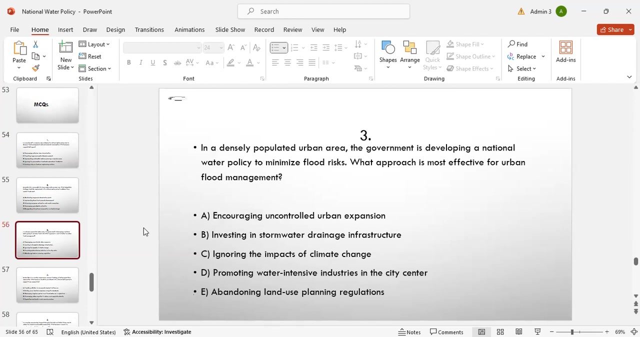 Option D is encouraging groundwater extraction. E is degrading international cooperation on climate change Anyone? Answer is option C: enhancing mangrove restoration and coastal ecosystem. MCQ number three is in our densely populated urban areas, the government is developing a national water policy. 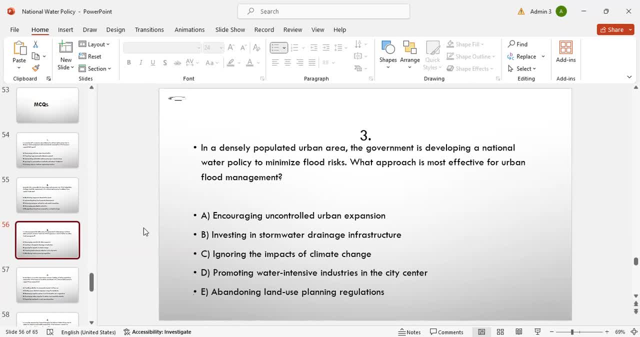 to minimize flood risk. What approach is most effective for urban flood management? Option A: encouraging uncontrolled urban expansion. Option B: investing in stormwater drainage infrastructure. Option C is ignoring impact of the climate change. Option D is promoting water intensive industry. 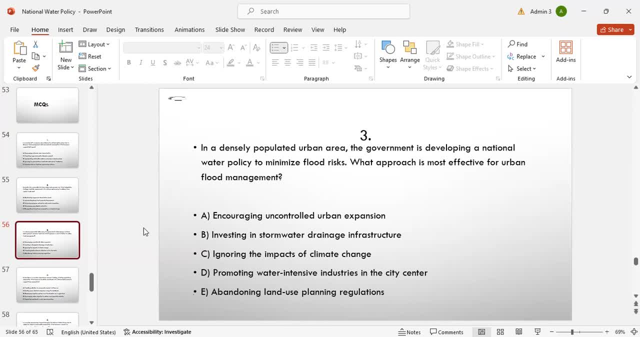 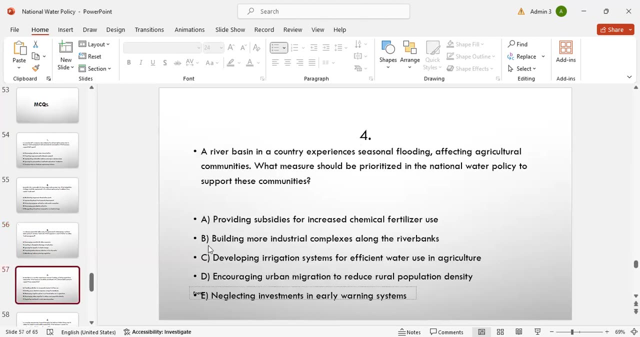 in the city center. Option E is abandoning land use planning regulation. Answer is option B: investing in stormwater drainage infrastructure. MCQ number four is a river basin. A river basin in our country experiences seasonal flooding. Effective agriculture communities. What measures should be prioritized in the natural water policies to support this community? Option A: providing subsides for increasing chemical fertilizer use. Option B: building more industrial complex along with riverbanks. Option C is developing irrigation system for efficient water use in agriculture. 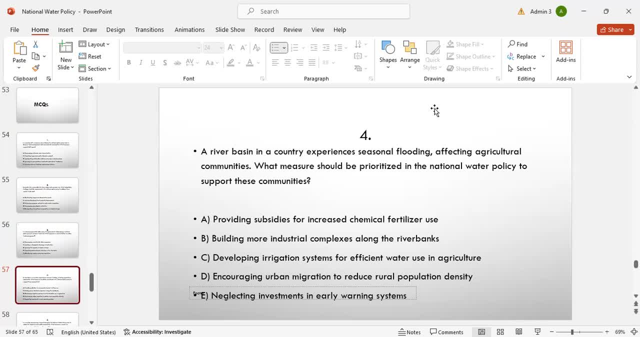 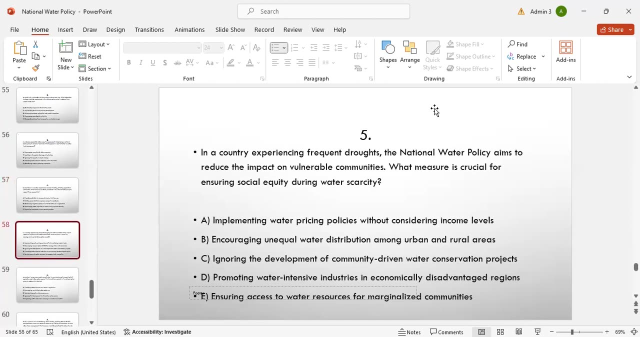 Option D is encouraging urban migration to reduce rural population density. Option E is neglecting investment in early warning system. Answer is option C: developing irrigation system for efficient water use in agriculture In a country experiencing frequent drought. the national water policy aim to reduce the impact on vulnerable communities. What measure is crucial for ensuring social equity during the water scarcity? Option E is implementing water pricing policies without considering income levels. Option B is encouraging unequal water distribution among the urban and rural areas. Option C is encouraging the development of the community driven water conservation projects. 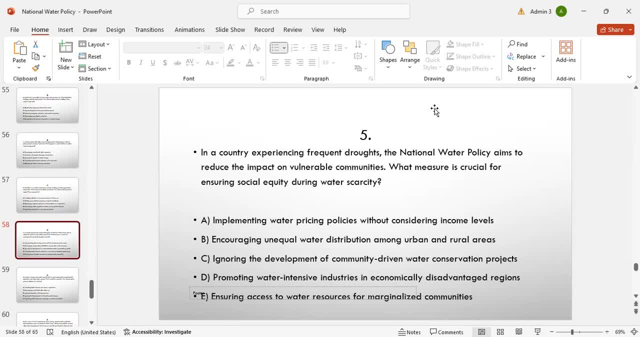 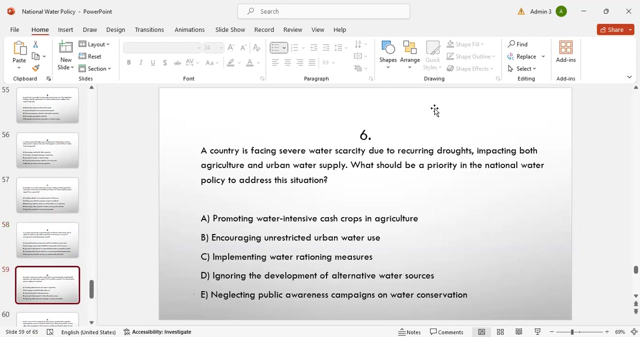 Option D is promoting water intensive industries in economically disadvantaged region. Option E is ensuring access to water resources for marginalized community. Answer is option E, ensuring access to water resources for marginalized communities. Our country is facing severe water scarcity due to the recurring drought impacting both agriculture and urban water supply. 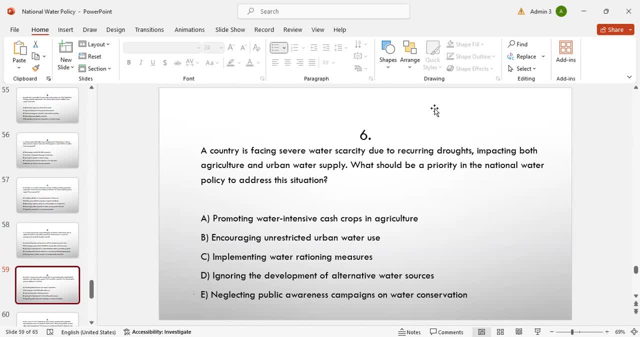 What should be a priority in the national water policy. Option A: promoting water intensive cash crop in agriculture. Option B: encouraging unrestricted urban water use. Option C: implementing water rationing measures. Option E is ignoring the development of alternative water resources. 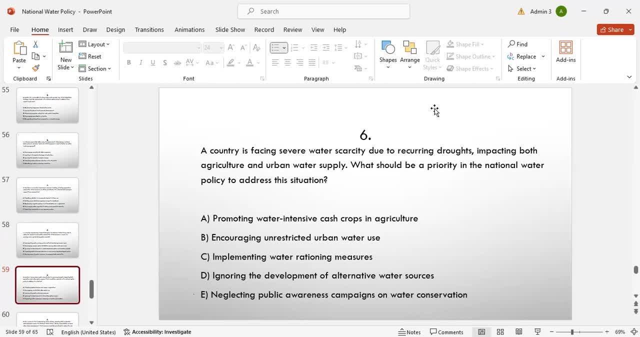 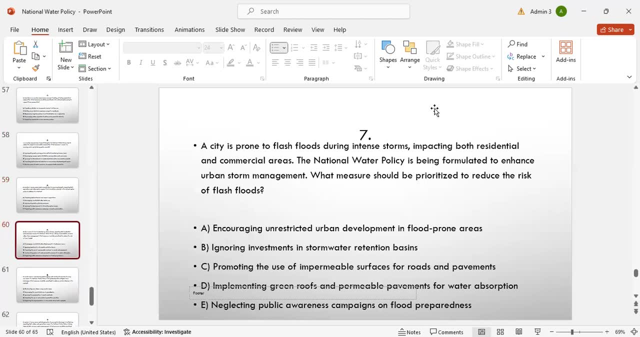 Option E is neglecting public awareness campaigns on water reservation. Answer is option C. MCO number 7 is a city prone to a flash flood during the intense storm, impacting both residential and commercial areas. The national water policy is being formulated to enhance urban storm management. 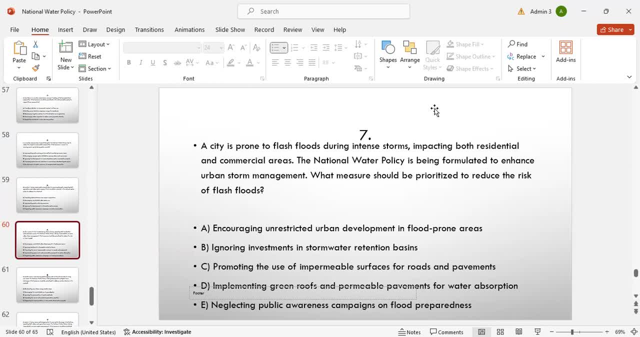 What measures should be prioritized to reduce the risk of flash floods? Option A: encouraging unrestricted urban development in the flood prone areas. Option B: ignoring investment in the storm water retention basins. Option C is promoting the use of impermeable surfaces for the roads and pavements. 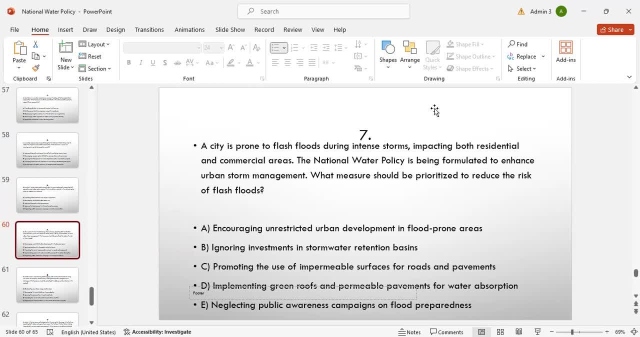 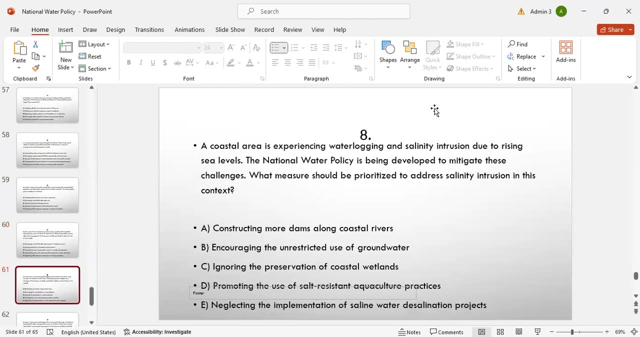 Option D is implementing green roofs and permeable pavement for water absorption. Option E is neglecting public awareness campaigns on the flood preparedness. Anyone Answer is option D. MCO number 8 is a coastal area is experiencing water logging and salinity intrusion due to rising sea levels. 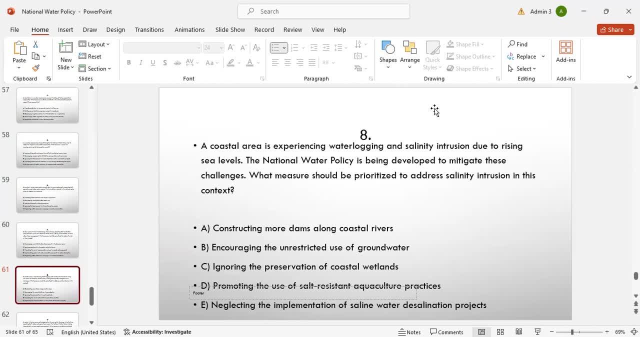 The national water policy is being developed to mitigate these challenges. What measures should be prioritized to address salinity intrusion in this context? Option A: constructing more dams during coastal rivers. Option B: incurring the unrestricted use of the groundwater. Option C: ignoring the preservation of the coastal wetlands. 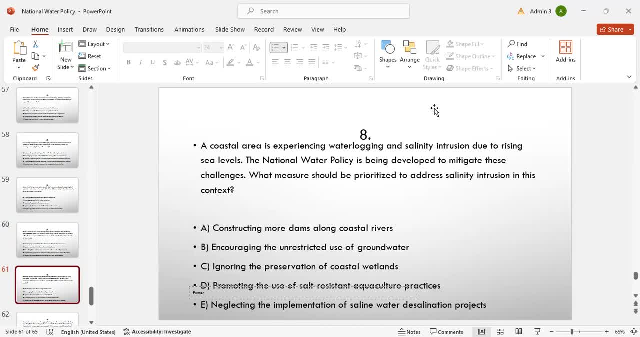 Option D is promoting the use of the salt resistant agriculture practice. Option E is neglecting public awareness campaigns. Option E is neglecting the implementation of the slime water desalination projects. Option D: promoting use of salt resistant agriculture practices. 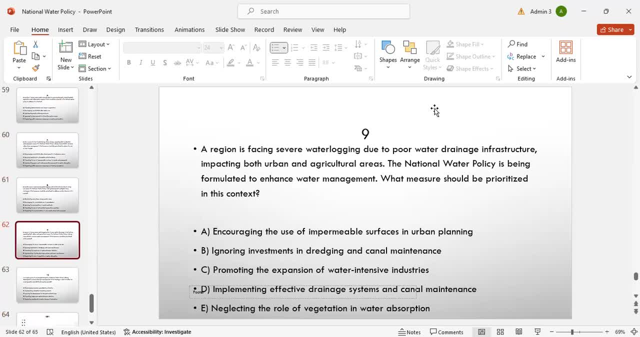 MCO number 9,. a region is facing severe water logging due to the poor water drainage infrastructure, impacting both urban and agriculture areas. The national water policy is being formulated to enhance water management. What measures should be prioritized in this context? Option A: encouraging the use of impermeable surface in the urban planning. 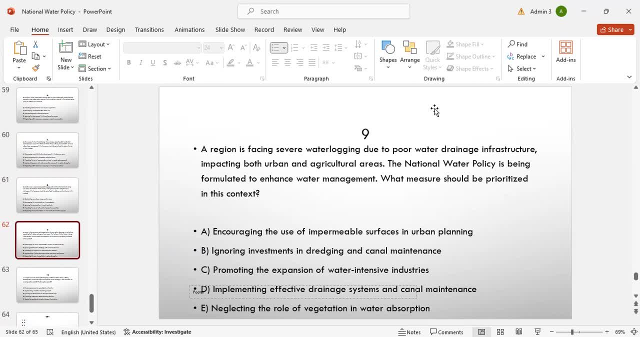 Option B, ignoring the investment of digging and canal maintenance. Option C is promoting the expansion of the water intensive industries. Option D is implementing effective drainage system and canal maintenance. Option E is neglecting the role of vegetation in the water absorption. 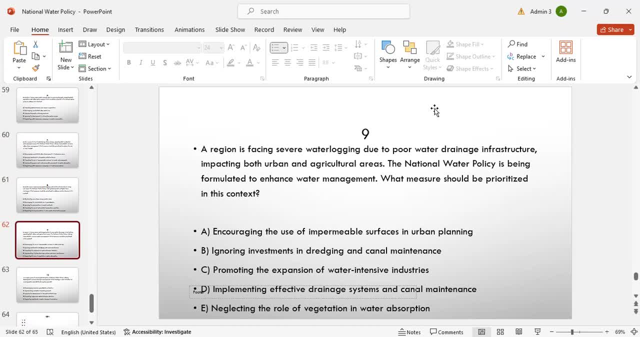 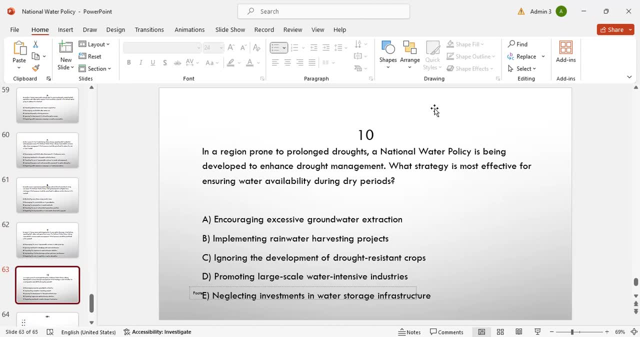 Answer is option D, implementing effective drainage system and canal maintenance. In our region, prone to the prolonged drought, our national water policy is being developed to enhance the drought management. What strategy is most effective for ensuring water availability during dry periods? Option A: encouraging excessive groundwater extraction. 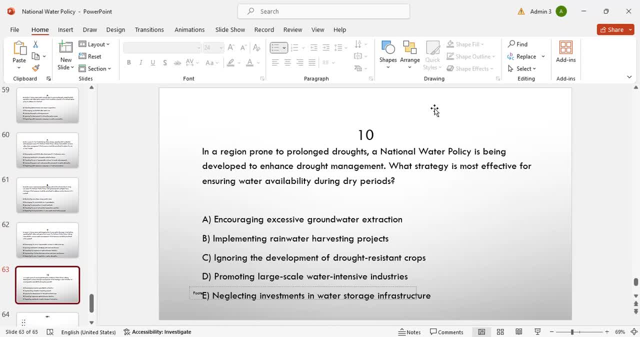 Option B: implementing rainwater harvesting projects. Option B- ignoring development of the drought resistant crops. Option D- promoting the large scale water intensive industries. Option D- neglecting investment in the water storage infrastructure. Answer is option B: implementing rainwater harvesting projects.